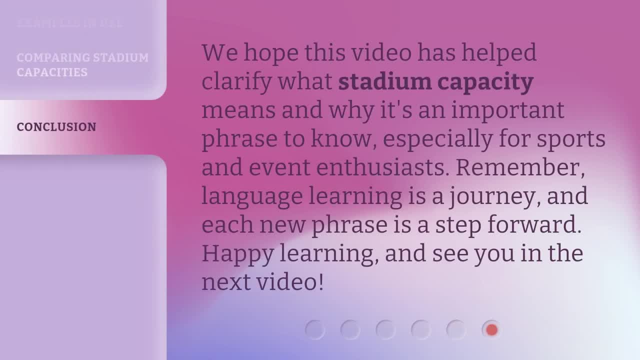 of the importance of stadium capacity. We hope this video has helped clarify what stadium capacity means and why it's an important phrase to know, especially for sports and event enthusiasts. Remember, language learning is a journey and each new phrase is a step forward. Happy learning and see you in the next video. 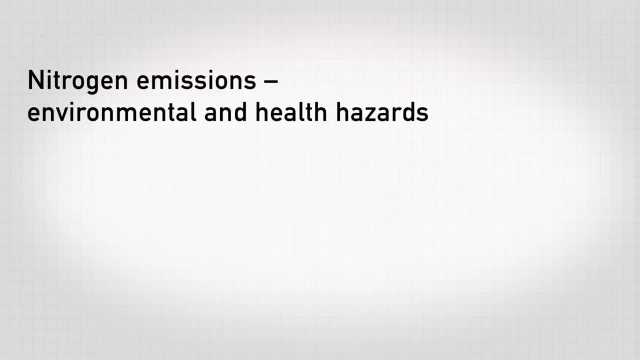 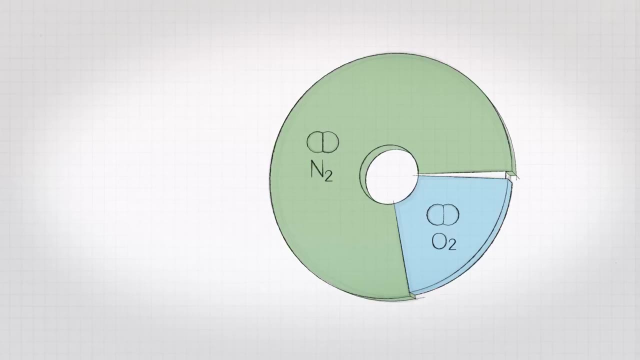 Nitrogen is abundant. 78% of the air consists of nitrogen in the form of N2.. This form of nitrogen is very stable, or in other words, not reactive. In addition, nitrogen is an essential element of all living beings, But before it is used by them, it has to be converted. 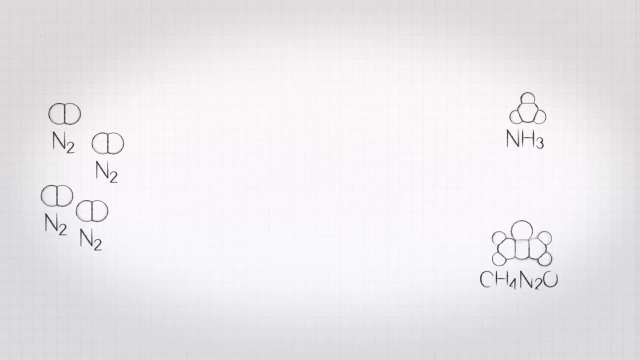 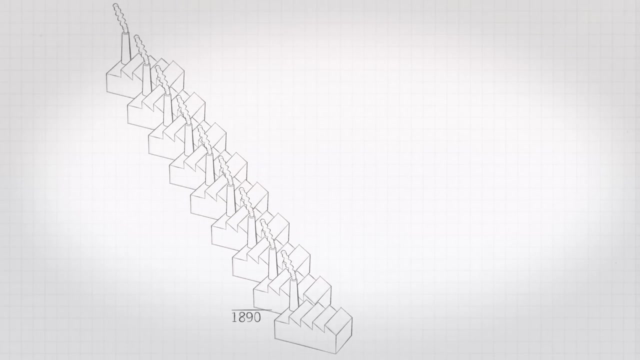 into reactive forms such as ammonia or urea. This can be done by specialised microorganisms or in large chemical factories. Since 1890, the yearly anthropogenic production of reactive nitrogen has increased ninefold. If too much reactive nitrogen is released into the environment, 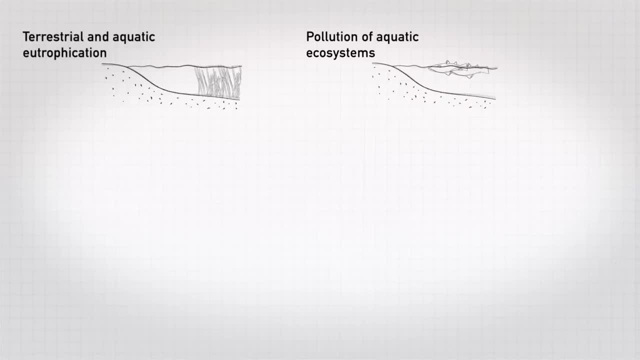 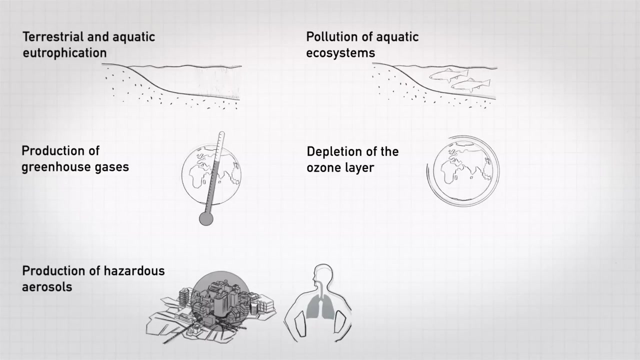 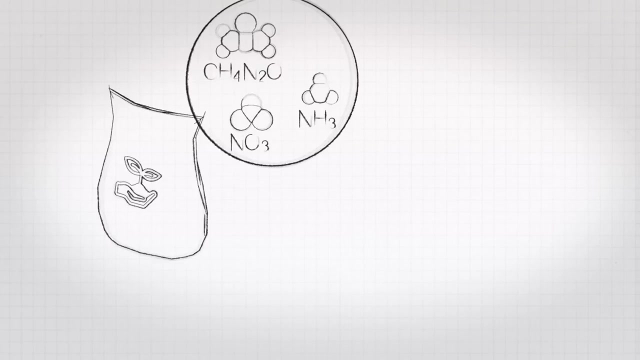 it can have many negative effects. Let's see how human excreta contributes to the harmful release of reactive nitrogen into the environment. Reactive nitrogen compounds such as urea, ammonia or nitrate are major components of fertilisers. They are applied to the soil to increase agricultural production. 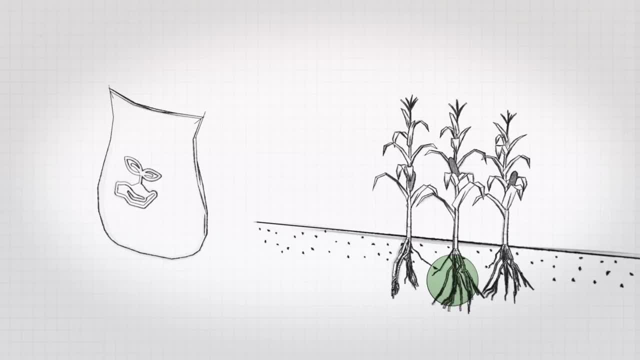 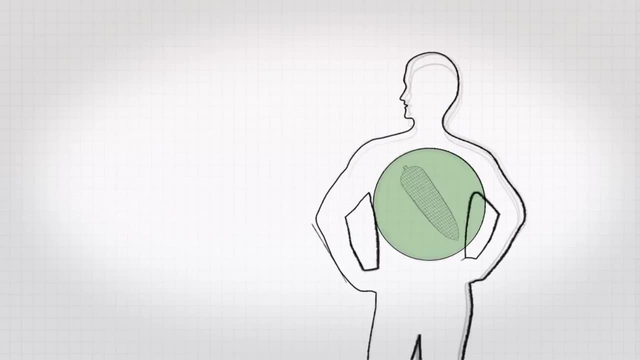 Plants need nitrogen to grow, and most plants take up reactive nitrogen from the soil. Humans also need nitrogen to grow. They need nitrogen to grow and receive it from the food they eat. A large amount of the nitrogen we take up as food is excreted in urine together with 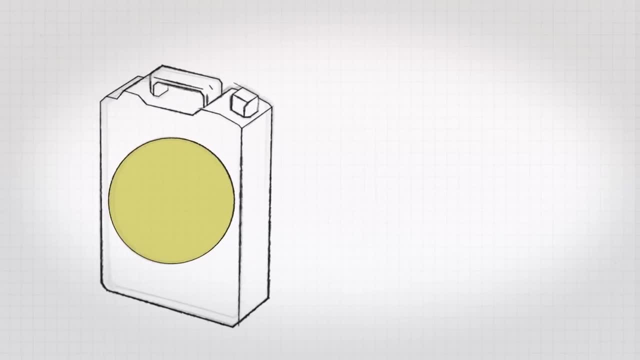 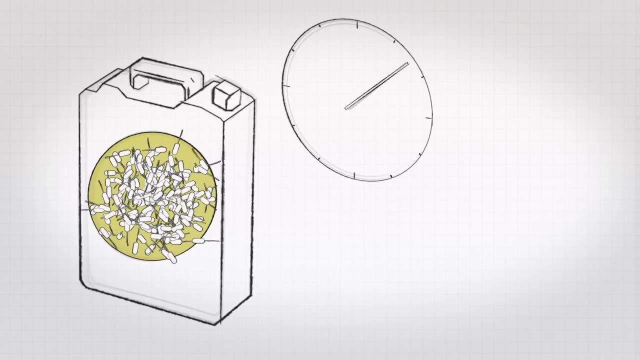 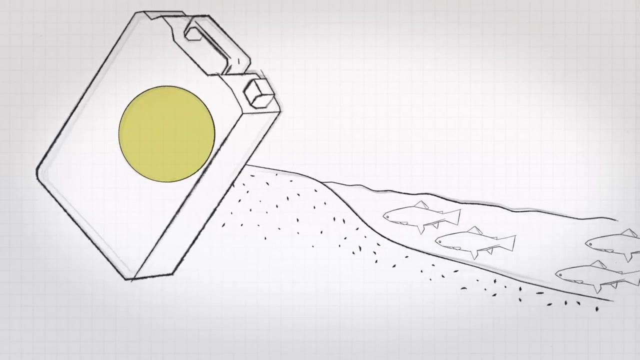 most of the other nutrients. In fresh urine, nitrogen is present as urea. When the urine is exposed to the environment, urea is spontaneously converted by bacteria into ammonia. When large amounts of urine or waste water reach open bodies of water, the high concentration of